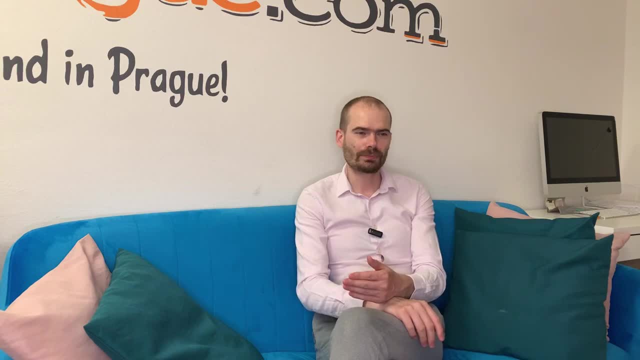 uh, it might be pretty difficult. it's possible. it's possible, but it might be pretty complicated. so let me just explain all the options. so the easiest way, or like almost the only one, but the the main one, the main way for bringing your family members to the czech republic. 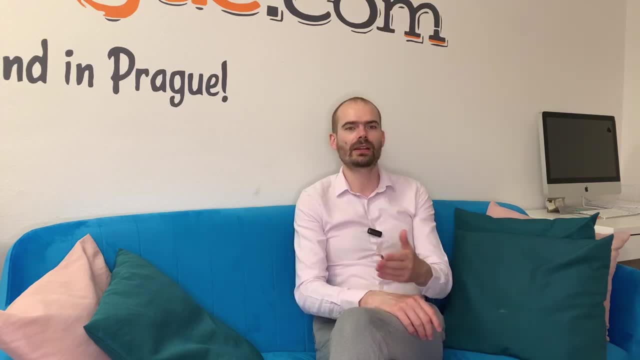 is through so-called family reunification visa or family reunification residence permit. i'll explain the difference in a second. but uh, it means that this visa or residence permit, this purpose of stay, is just to be with the family members. so let's say, you are the main applicant. 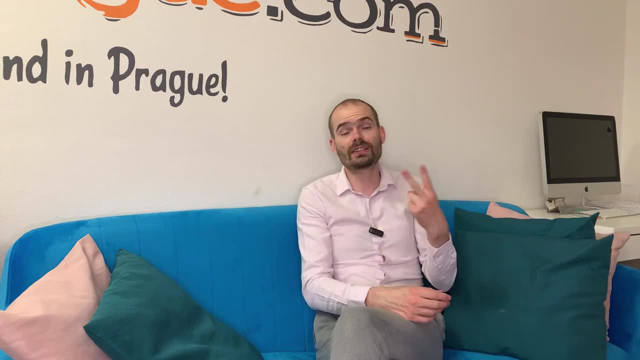 you already have here, like an employee card or even a student visa, student residence permit, or blue card or business visa, business residence permit, it doesn't matter. basically, whatever type of visa you have, uh, you can bring your family. so because we get this question often, like, hey, i'm a student, can i bring my spouse or kids? you can, as long as you meet all the other. 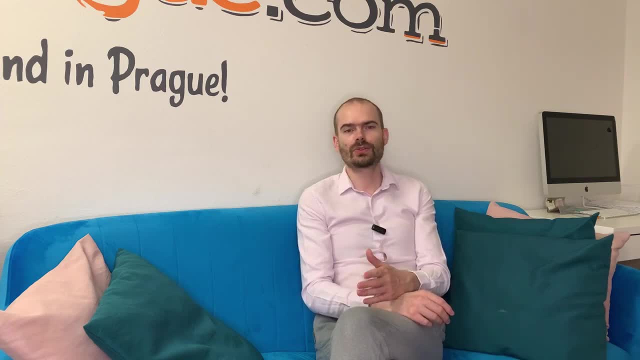 conditions because there are some like money requirements. so as long as you meet those, it doesn't matter if you have a student visa or residence permit or business visa- business residence permit, employee card, blue card, whatever else- you can always bring your family. so the easiest way to do that is through a long-term visa with the purpose of family reunification. 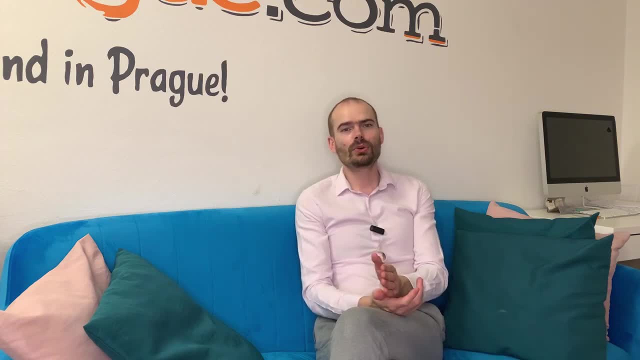 why it's the easiest is that you only need to show that you have enough money in your bank account. so basically, anyone can apply as long as you have enough money in your bank account. but, for example, for the residence permit, which is the other option, you need to show that you are making. 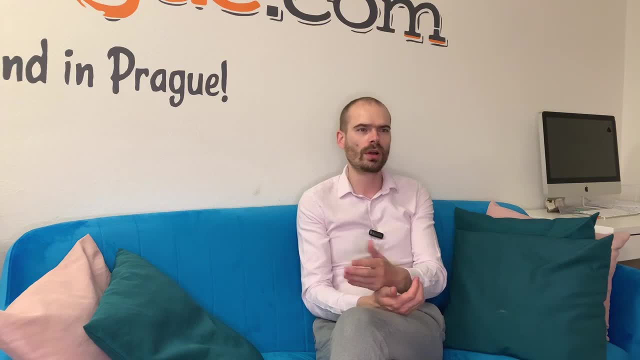 enough money on monthly basis. so, for example, if your salary is low or if you're a student and you don't have any income, then the easiest way is to show that you have enough money in your bank account just through the long-term visa with the family reunification purpose of stay. another question: 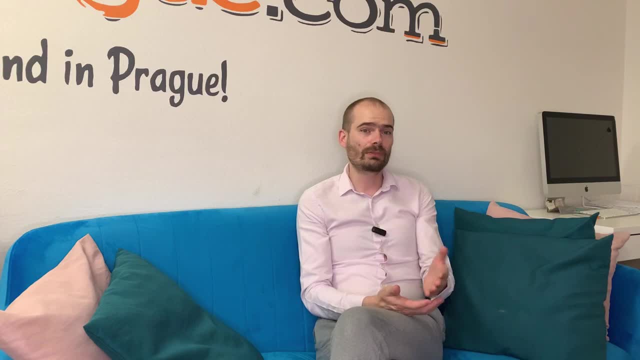 we get often, or one kind of misconception or something which is not understood properly, is that people think that you can only bring your family after some amount of time, like after 15 months or something like that. that's not true. you can bring your family immediately under the 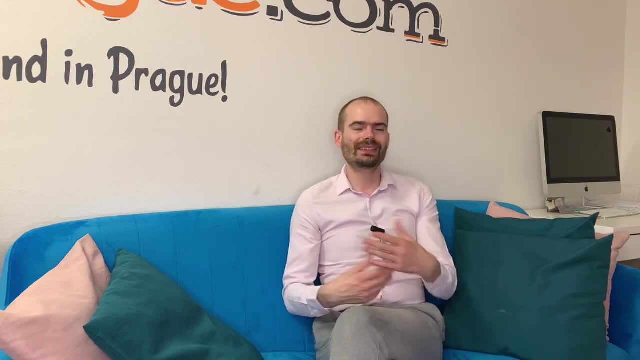 long-term visa. if we talk about the long-term residence permit, that's a different story and there are some rules for that. but if you want to bring them under the family- family reunification visa, you can do that anytime. so technically you can apply all at the same time. so the main applicant applies for. 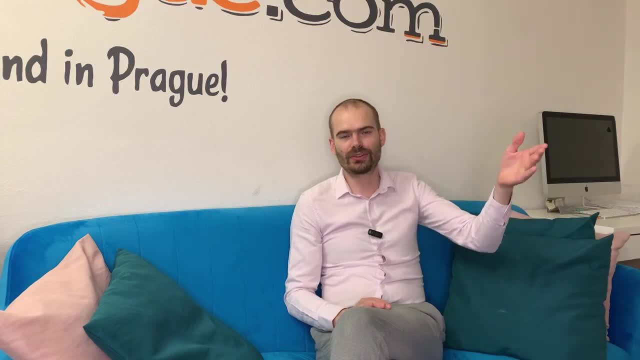 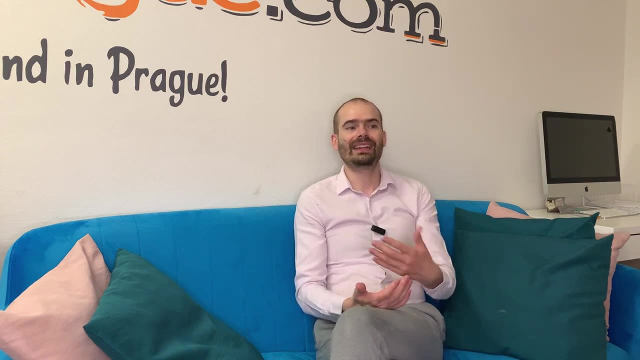 an employee card and his or her spouse and kids can apply at the same time the same day at the embassy. you can all apply at the same time. there's no problem with that and in some cases it's the best way to do that. of course, in some cases it might be better to first get the main applicant. approved, because then the family is kind of like: sure, nothing is sure with the, with the czech immigration. that's why i do this, but it's very likely to get the family here as well. in some cases it's better just to apply: all together, so you can come all together, so that's. 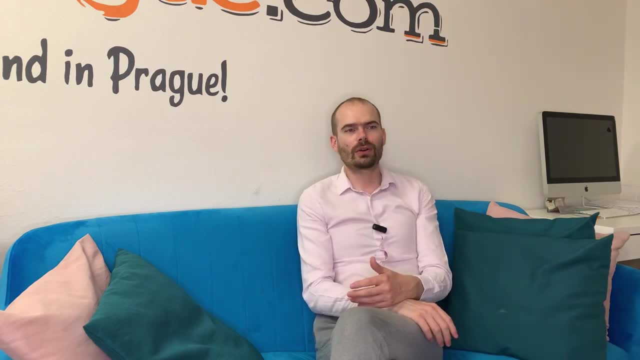 the long-term visa with the purpose of family reunification. the main conditions there are, of course, like you need to be a family member, so spouse kid parents. in some very limited cases, you need to show that you have enough money in your bank account. as of now, it's equivalent to. 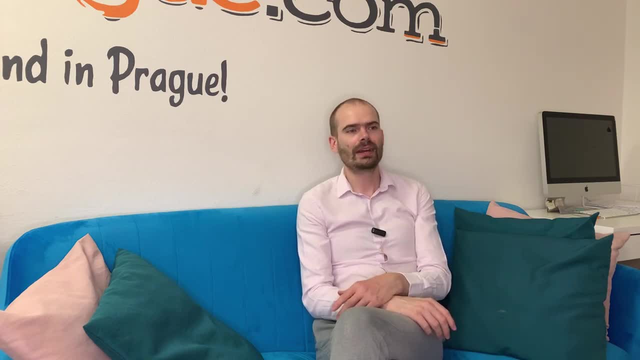 120 000 crowns for an adult person. kids usually need to have half of it, so 60, 60 000 crowns. but if you have enough and you can prove that you are family members- meaning you have your marriage certificate, with apple, steel, super legalization and everything- and if you have the birth certificate, 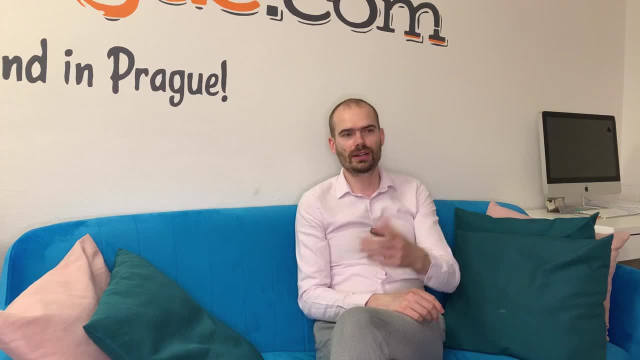 for kids, for example, that they are your kids or that you are their parent. uh, apple steel super legalization. translated into czech, you can apply for the family reunification visa. the family reunification visa is a sticker in their passport, valid for up to one year. doesn't allow them to work. i've done a video about the difference between the long-term 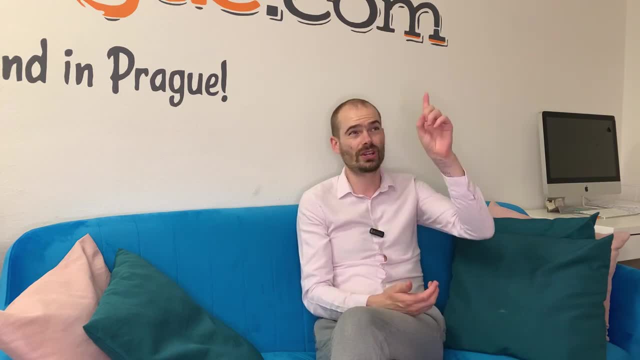 visa: residence permit when you can work with when you cannot work. i will share it somewhere here, i guess. so this video is not about that. it's just about giving you the the idea how it all works. so then, the second thing that you need to do is to apply for the family reunification visa. 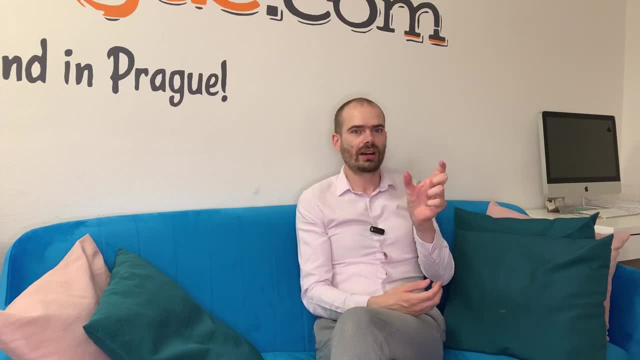 so the second option would be a long-term residence permit, which is like the biometric card, but you can only apply for that if you have, if the main applicant has been living in the czech republic for long enough. so, for example, for a blue card it's zero days or zero months, so you 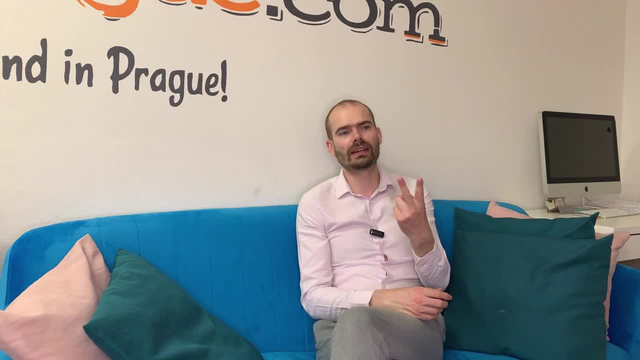 can all apply together. the main applicant for a blue card and your family can apply for a long-term residence permit with the purpose of family reunification. for employee card holders, it's six months and for all the other purposes, so students, the other visa or business residence permit, it's 15 months after the main applicant has been living here. 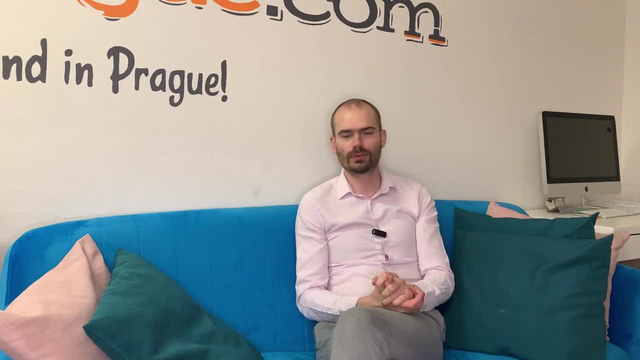 so that's probably what people are confused. so, or what they are confused about, like that you cannot bring your family after some amount of months. that only applies for the residence permit application. with the visa they can come anytime. um, yeah, but one of the main things for the residence permit or 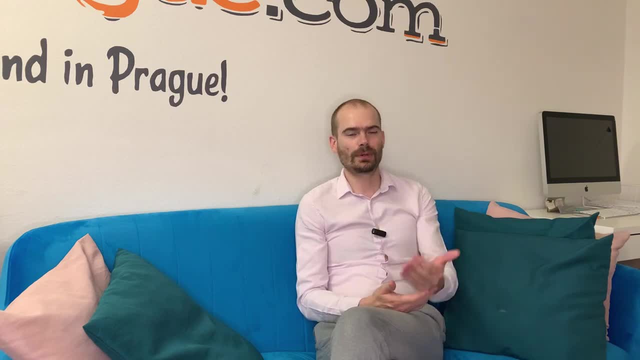 where people sometimes have problems is that for the residence permit- you can apply for a long-term residence permit- you need to show- or the main applicant actually needs to show- that you are making enough money on monthly basis to cover the whole family. so if you're a software developer or like a manager or 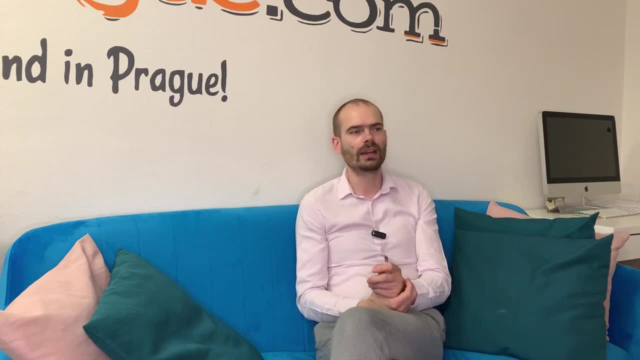 like some, you work in some big international company. uh, you should be fine and you will most likely meet the requirements. because, let's say, for a family of two the required income would be roughly, let's say eight plus eighteen, so twenty six thousand. the net for a family of three that would be twenty two plus twelve, let's say so thirty six thousand crowns. so 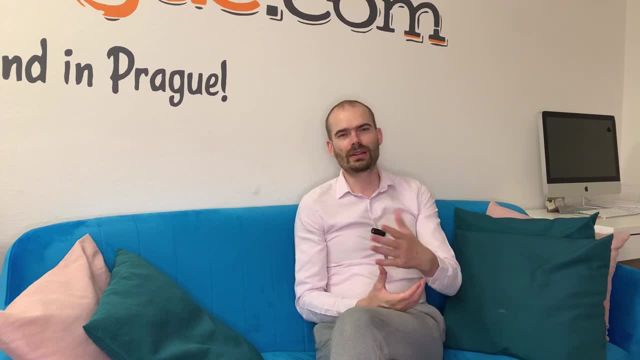 you should all meet this requirement. but if you, for example, work in a restaurant or somewhere where, where you have like the minimum salary in your like pay slips, uh, or in your contract, and then you get some money- uh, in cash, unfortunately you might, you might not qualify, or your family. 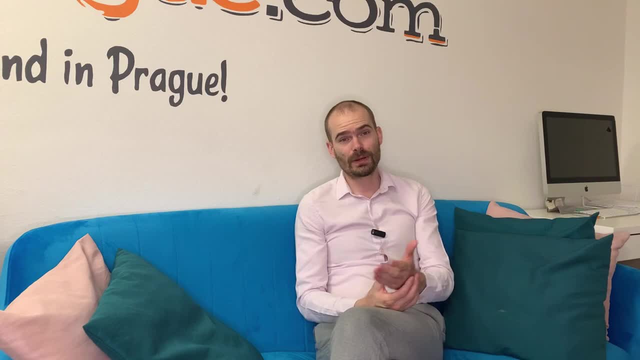 members might not qualify for the residence permit because you need to show that you have enough money coming to the, to the household, on monthly basis, um, so there are ways around that. if you want to know about those, get in touch and i'll be happy to discuss that in person. but generally, for the residence permit, you need to show that you have enough money in your uh that you're coming in to the household every month so that you have high enough monthly salary. in some cases, family members can also apply directly for permanent residence permit, but that only, or primarily applies. 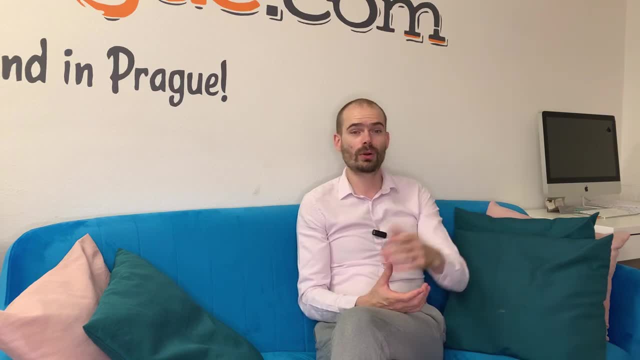 then usuit it for permanent residence permit. but that only, or primarily applies applies to kids- if the main applicant, the parent, already has a permanent residence permit in the Czech Republic. We are now just finishing a case with an Indian client whose daughter just came to the Czech. 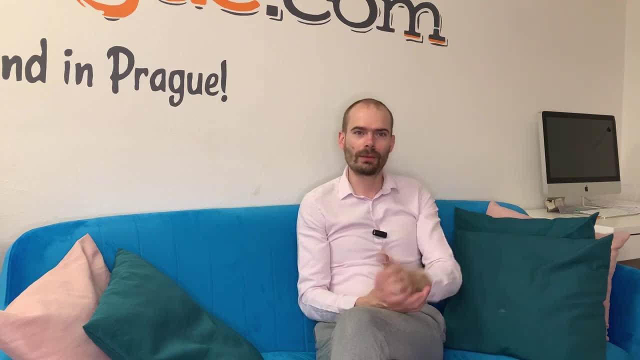 Republic today, earlier today, and we applied for the permanent residence permit directly. So she will be like it's her first day in the Czech Republic now, today, and she will be picking up her permanent residence permit, let's say, a month from now, after she gives. 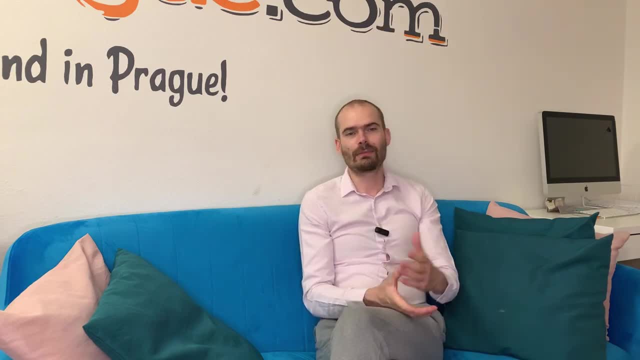 the biometric details and picks up the card. So that's an amazing way for kids to get set in the Czech Republic. So these are the main options, And then one option for the couple that are not married, because we've had a couple questions. 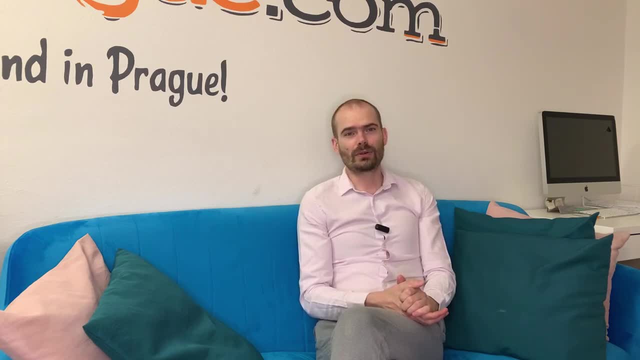 about that recently as well. So if you're not married and you are both non-EU citizens, if you're EU citizens, you can apply for the partnership visa. If one of you- One of you- is EU citizen, one of you is non-EU, I will share the link here as well. 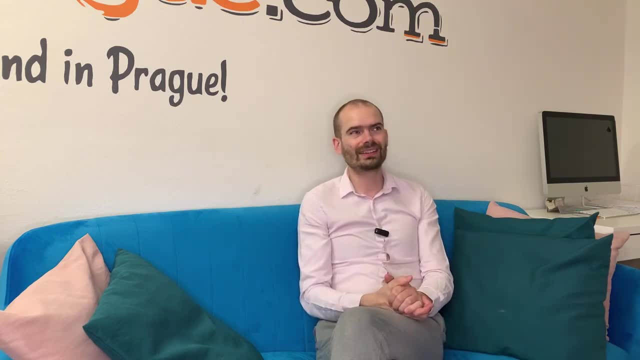 But if you're both non-EU citizens and you are just dating, you can try the other purpose of stay, because there is this other purpose of stay or other type of visa which you can apply for if you don't fall under any category. 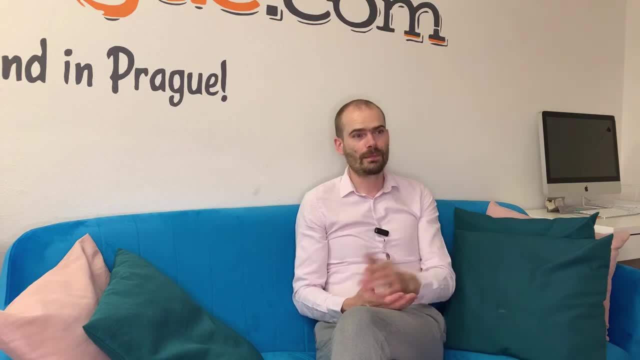 So if you don't fall under the family reunification because you are not married, then you can still try and apply for the other purpose of stay. But we cannot guarantee anything there because it's totally up to the decision maker. and if they are fine with you coming here and if they believe that you're a real couple, 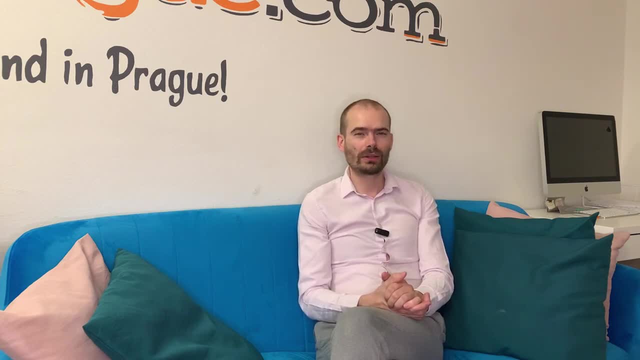 or not. So of course you should be. I would only recommend doing this in case you've been together for a very long time, like at least couple of years. You have proofs of that. You lived together maybe, or maybe you have the civil marriage or you have like. 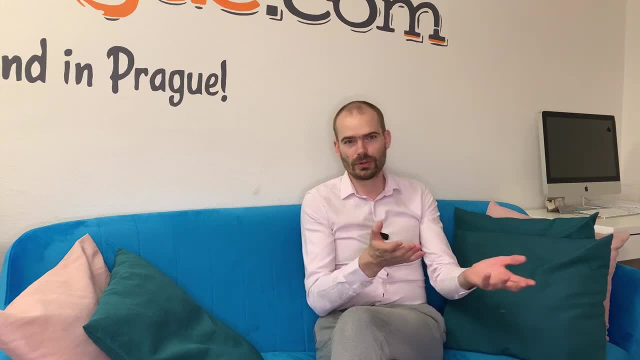 You're a gay couple and you have. You cannot get married in the country where you're from, But you have some kind of registration Or something that you can prove that you have really been a couple, that you really lived together, that you traveled together, all that. 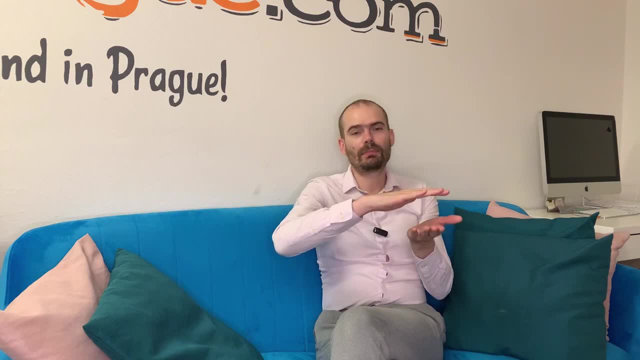 So if you can prove this and you can submit this big pile of documents to the embassy, you can try, And I've seen it happen. I've seen it happen, maybe like three times. That's not a common way of dealing with the visa, but I've seen it happen.